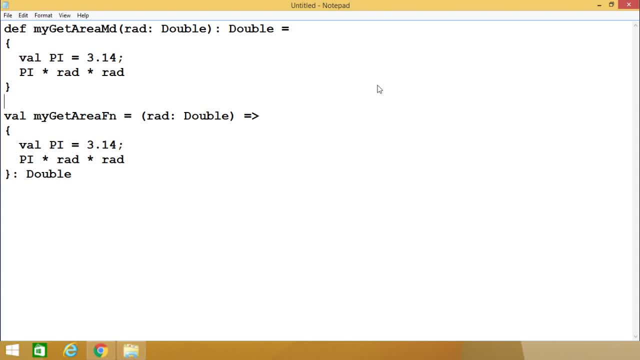 this respective implementation of the method and the functions in our Scala programming. So at first we are considering this respective Scala method. So methods are not objects and the term method and object are often used interchangeably because Scala functions are when methods are the 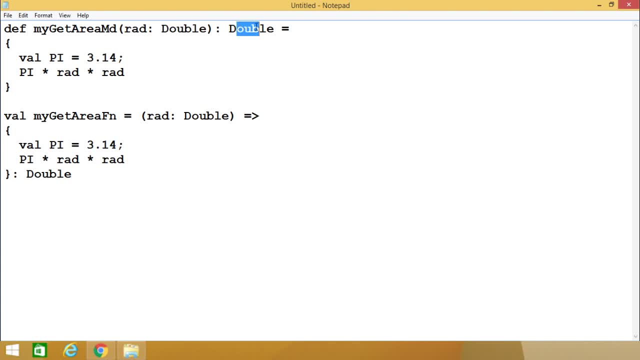 intended object. The term method is the theft words, which means theedy swear words, or you can use it any other way you like. In the overall mode, in the Basically class and in Scalar programming method are two types of method today. the first one is the CIFD method. 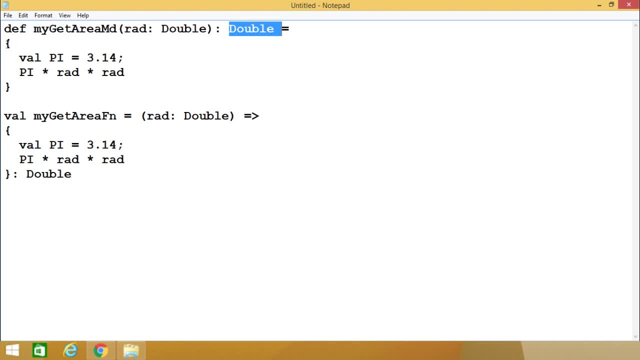 which is the 59V method, which is known as the First Private Phased method, and the last is the dolomite method output argument. it returns a double as output argument, so it is a body and which has been enclosed within curly braces and there is one equal to symbol is there and this is a body of. 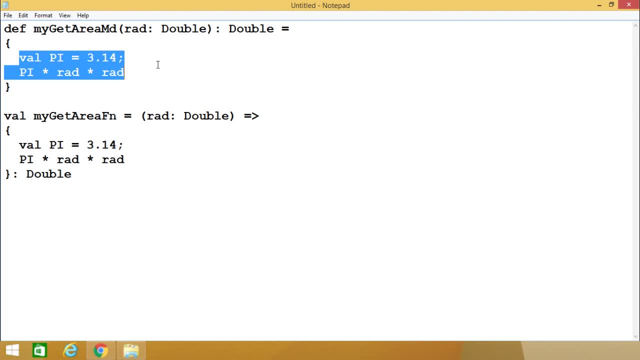 the method. so that's why we have defined that methods are not objects and the term method and object are often used interchangeably, because methods can be stored in objects quite easily and this method depicts the behavior of a class or an object. so now, if you go, if you consider the 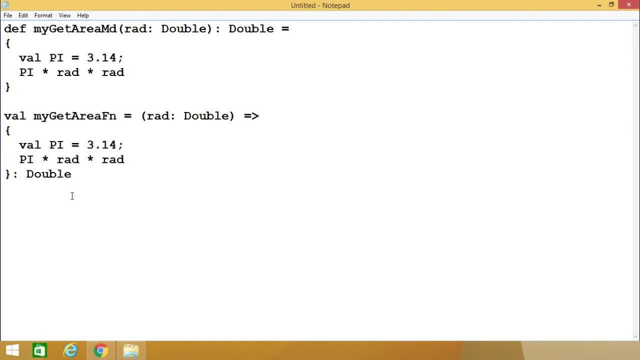 function. so functions are objects and function objects are first class entry entities on par with the classes, and methods are not like these objects. so whenever we are going to define one function, then it will be starting with the keyword val or var. so here you see, here we have defined. 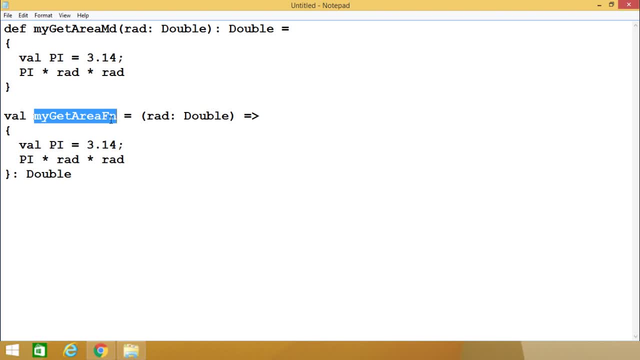 this one is the name of the function. there is a my get area function is equal to rad colon double. so it takes one input argument of the type double and it returns, say here. you see, here it is equal to symbol, but here we are having this arrow. 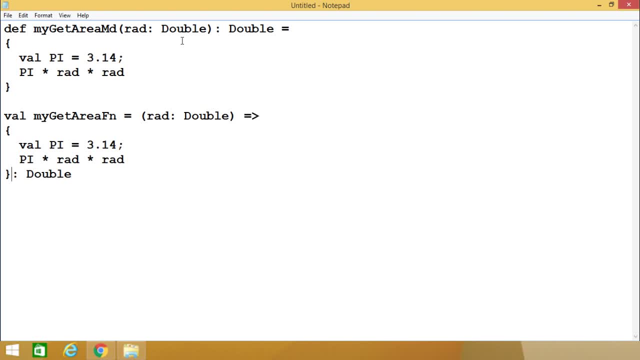 and this is a respective function body. and here we wrote the return argument like this one, return type like this one. but here we have written the same with some different syntax. the body is same, that means like this one. so what will happen if we want to write this respective method? so i must. 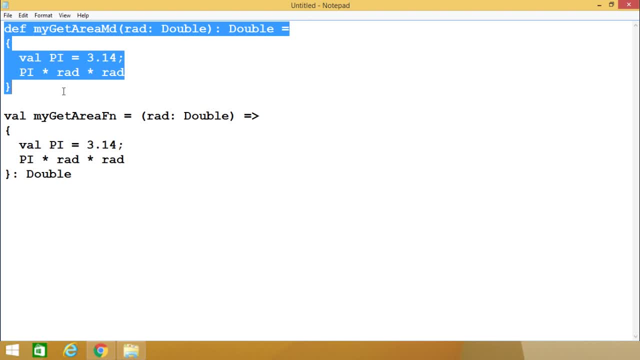 be writing this one a under one class or respective object. but in case of repl that means in case of directly in the shell, that is a scholar shell. if you write this particular method, so that is no need to write it in the respective class or object. we can write it directly in the in the interactive. 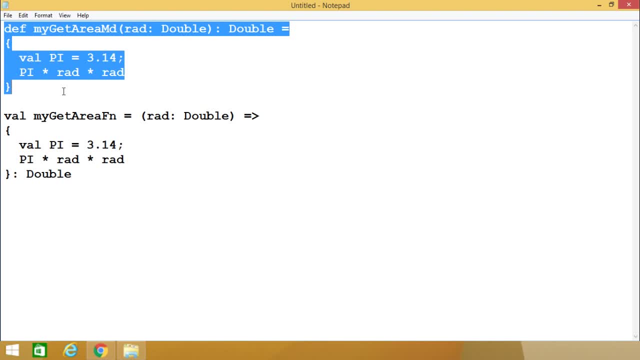 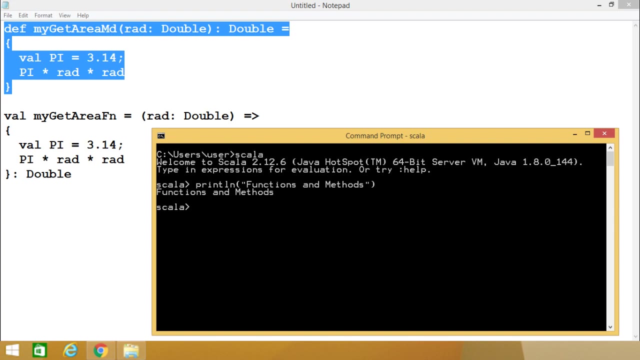 mode and that is known as the repl mode. so repl actually. you know that repl means the read evaluate print loop. so that is a repl. so that means, this is the repl. so here we can write our code, here we can write our respective programs and we can execute it. there is a interactive mode here and this repl is also. 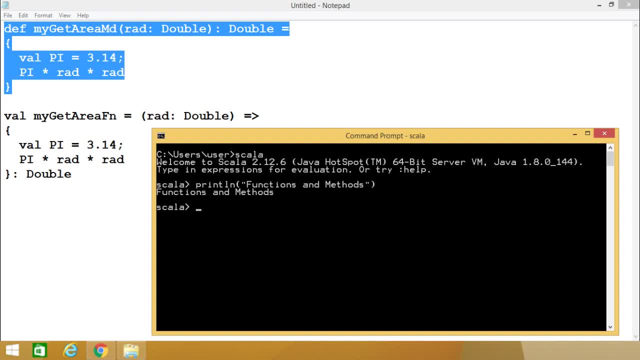 known as an interactive top level or language. shell is a simple interactive computer programming environment that takes single user inputs, and that is, a user expressions or single expressions- and evaluates them and returns a result to the user. a program in a repl environment is executed piecewise and we know that in case of methods, the methods are. 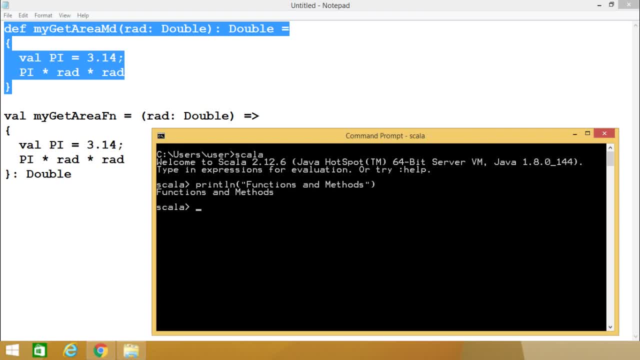 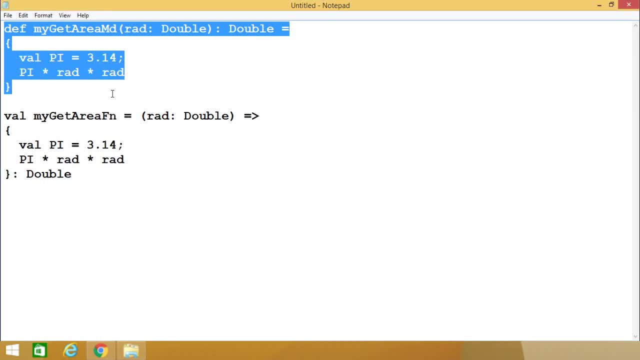 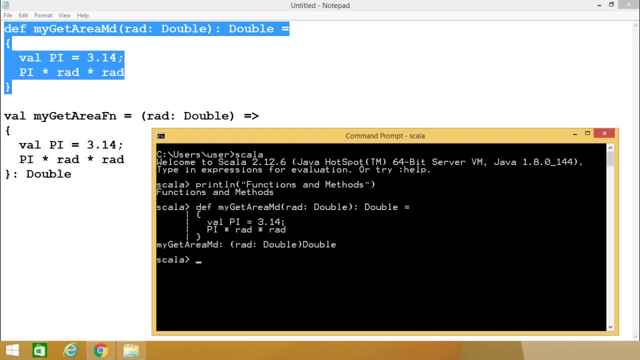 to be written either within the class or within an object, but this method can also be written directly into this repl, so let me copy this one, let me copy it and let me do the pasting and pressing enter. now you can find that one method has got defined. the name of the method: 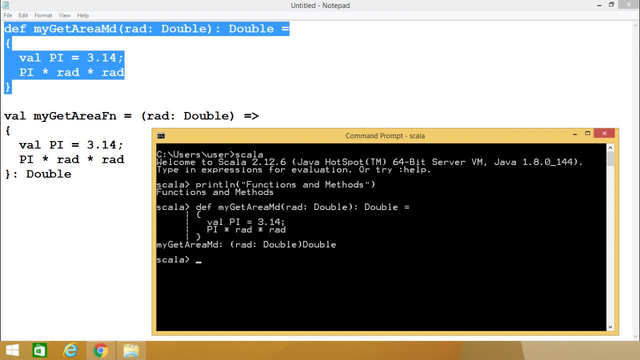 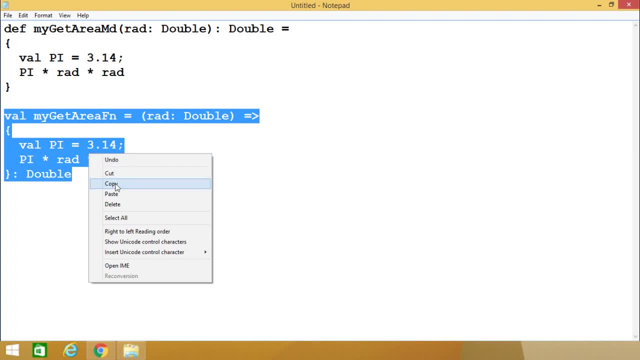 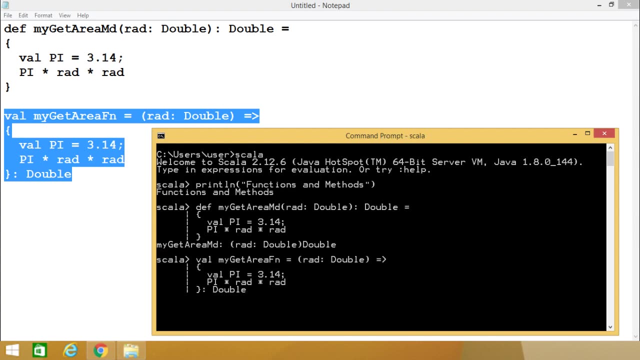 has been given and it is taking one red as input argument of the type double and returns double. so this particular function can also be done, the copy and paste here. okay, so now here you see, the name of the function has been given which takes this double as. 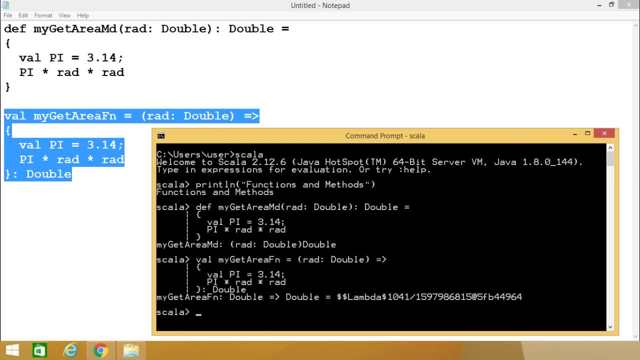 input double as output, and these are respective reference of this particular and this particular object, whatever has been created. so let us discuss more into details about the differences between the functions and the respective methods in our Scala programming. so functions, it is actually returning a value. that means it value types. 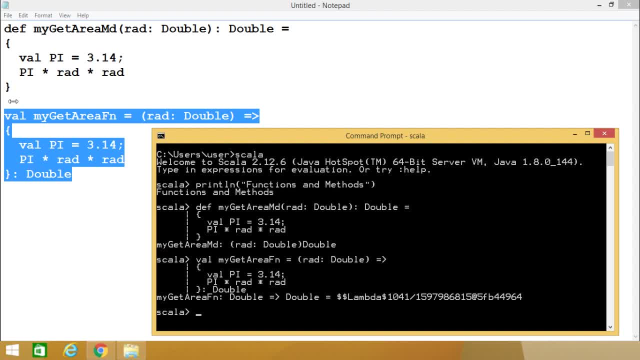 and can be stored in Val or bar storage units, as we have mentioned here already, and methods. that means that it is not the value type and cannot be served as a R values. that is, a right-hand side value or R value can be or cannot be defined using this. can only be defined using the def. 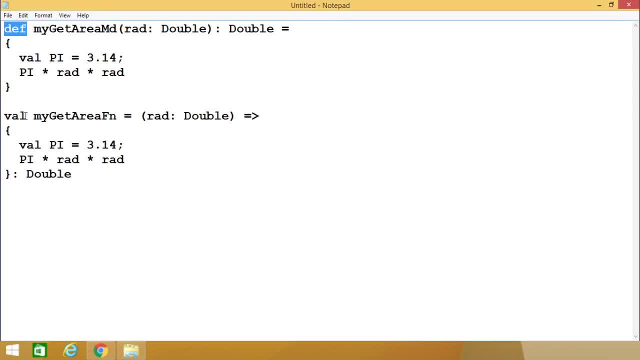 as we did this one. so there is no need to put, there is no scope to put any val or var against the method declaration. so here we'll be defining here this method using this def keyword, that is, the definition or define, if you consider the other differences between these functions and 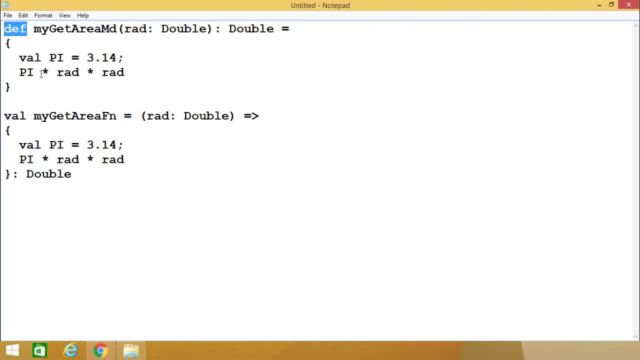 methods we can consider that functions are slightly slower and because it is having higher over it, because there are multiple indirections are there in case of functions, but on the method if you consider they are slightly faster and better performing. and in case of function they don't accept type parameters or parameter default values, so that are not available in case of. 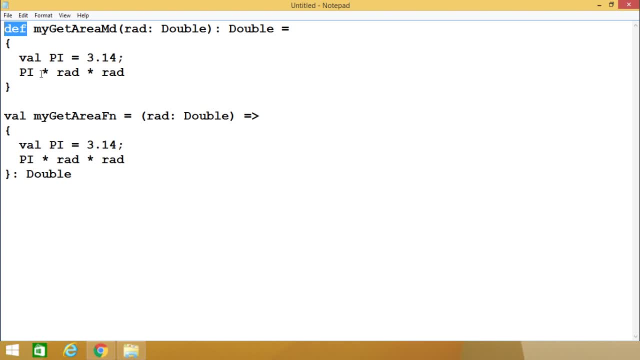 functions- and regarding this, we'll be having a separate video for the more discussion about these default values and all. but in case of methods, it works fine with the type parameters and the parameter default value, so that scope is available only in case of method. so methods are associated with a class and functions are not. 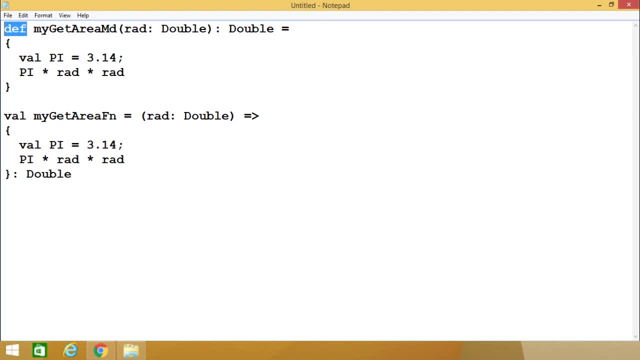 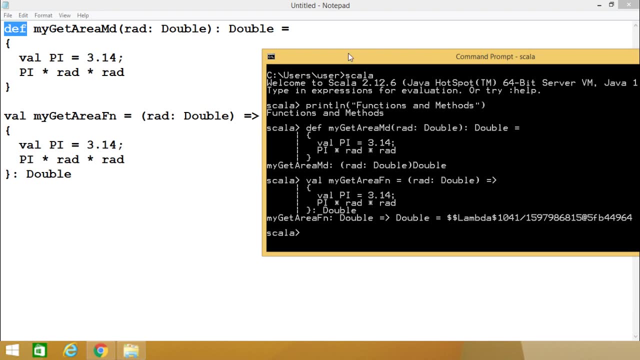 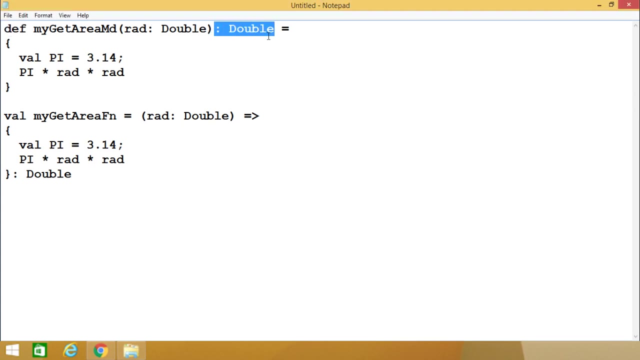 associated with a class or object. so now we have defined both the methods and the classes here. so now let me execute the same. so let me repeat once again what are the basic difference between their constructions? here you see, the output argument has been written in this way in case of method. 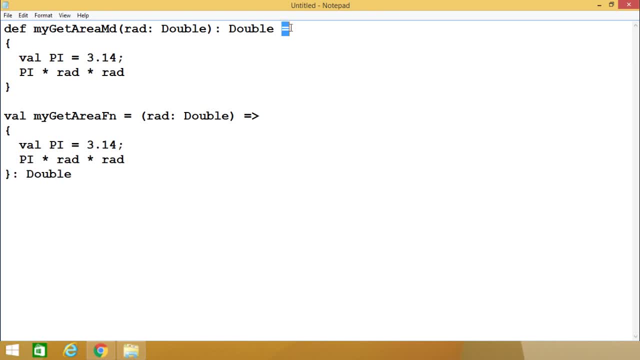